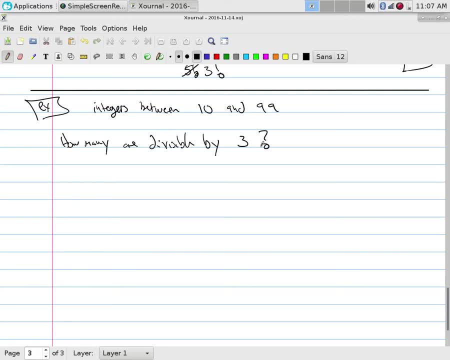 So all numbers, right, all numbers have a remainder of zero, one or two when you divide by three. So that would tell us that if I would say the infinite numbers- there are, a third of them are divisible by three, They have a remainder of zero, A third of them have a remainder of one And a third of them have a remainder of two. 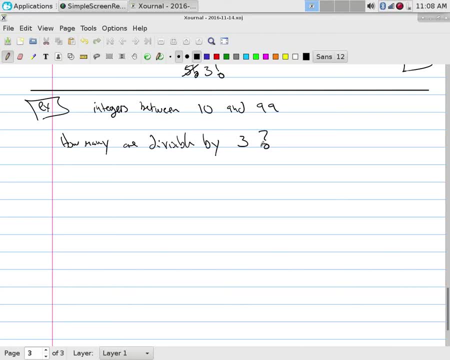 Does that make sense? So if I had an infinite amount of numbers, a third and a third and a third are divisible by three. What if I said divisible by seven? How many would be divisible by seven, One seventh, And then how many would not be divisible by seven? 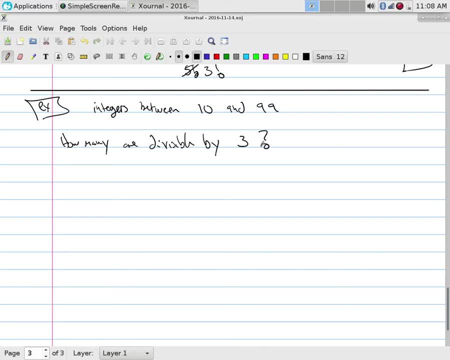 Six sevenths, The other, like one seventh, would have a remainder of one One seventh would have. well, just put them all together and just say six sevenths. if I say not divisible by seven, Okay, So divisible Divisible by three, normally is a third, right, It's normally a third. 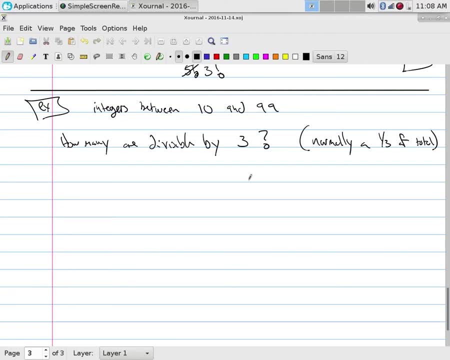 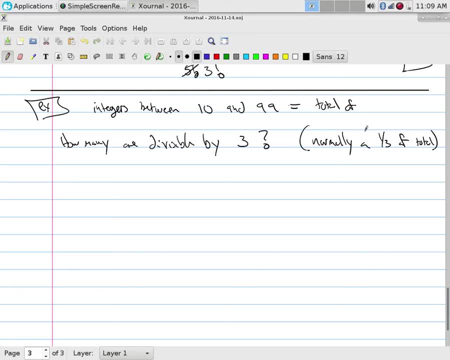 If we subtract, I would say, let's say we do one, two and three and four. Why don't we include ten and nineteen? Yes, we're, we're, oh, between and including. It's one of the things. if there's ever a doubt in what I say, ask specific. if there's ever a doubt when you're talking to somebody like did you mean to say something? 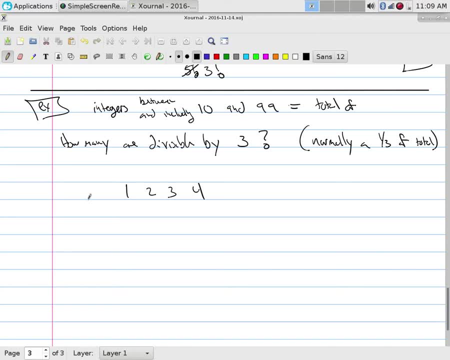 Because between would actually be what? Not eighty-nine, but eighty-eight Right. If I include it, it's going to be what? There's ninety of them, right? Eighty-nine plus one, because the first is your zeroth right. 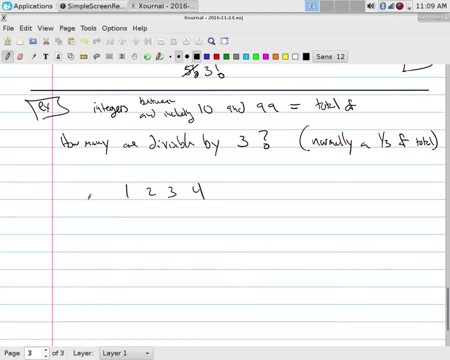 Like for example here: From one to four, If I take four minus one, I get what? Three, Three. But that means there's actually three, That three. what did you really count? Four minus one, I get what. 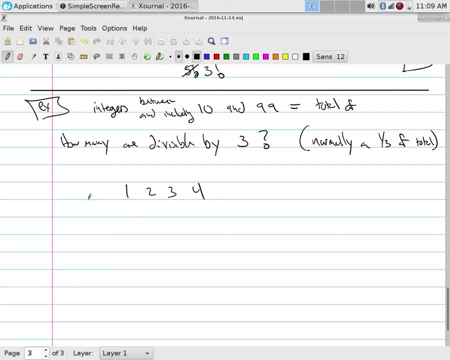 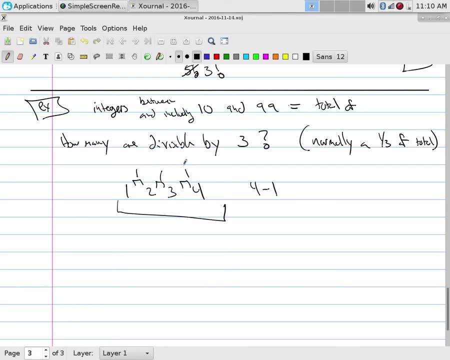 The gaps. When you subtract the ends, you get the gaps. So how many numbers are there? Gaps plus one Right, Which will take you back to four numbers. But if I said strictly between, do I really mean two, which is Gaps minus one? 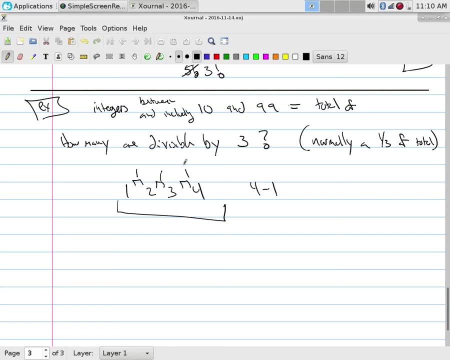 And so it's one of the things. when you said between, did you mean between including the end points Or not? You said if you mean including the end points, like for one to four is four. if you said not the one, you meant three. if you said gaps, you mean three if you. 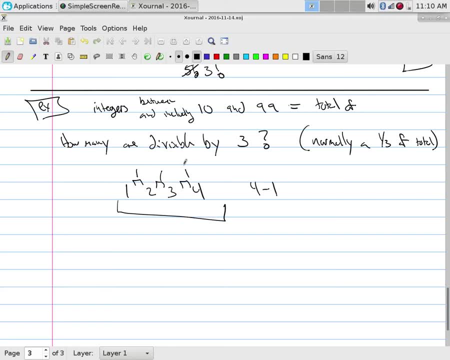 mean between, between and not the endpoints. then you mean two. so for us I meant including the endpoints, and so we have a total of 90. so if I gave you 90 sequential numbers, how many are divisible by three thirty? how many are divisible by four? normally it would be what one-fourth of total? 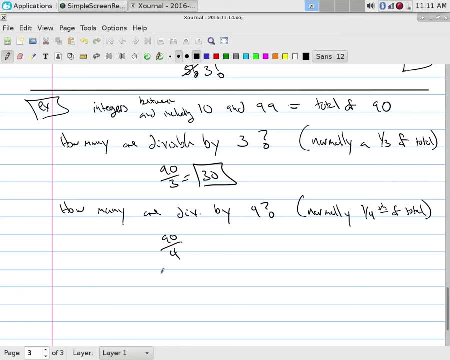 but what is 90 divided by four? what's half of 90? what's half of 45? hmm, half of 45, 22.5. all right, now we have a problem. in other words, this wasn't an exact multiple of four. so what this is going to is 22.5 tells us what there are. 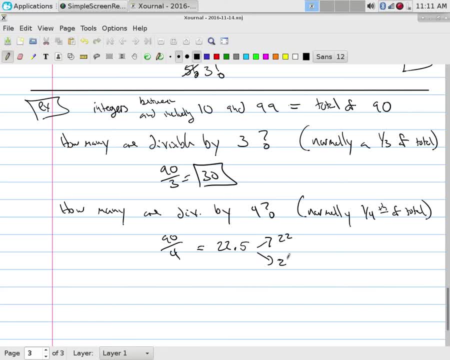 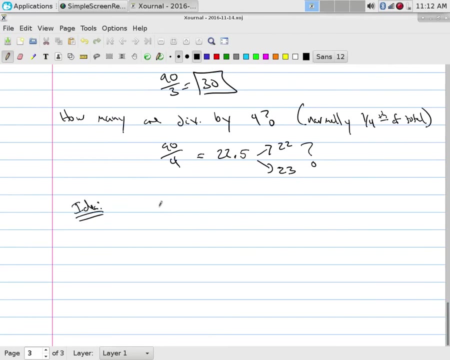 either going to be 22 or 23. there are going to be 23. we got to figure out which. all right. here's the idea for the numbers. say one, two, three, four. right has what we have: four numbers. if I say div by three, what's four divided by three? that is one point. three, repeating: 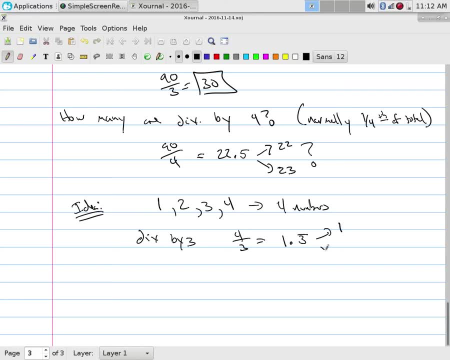 right, which means the answer is either going to be one or it's going to be two. for these numbers between one and four, how many are divisible by three? for one to four, it is only going to be. it's this because it's only. we have only three. 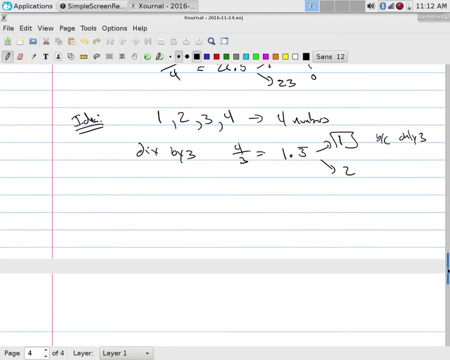 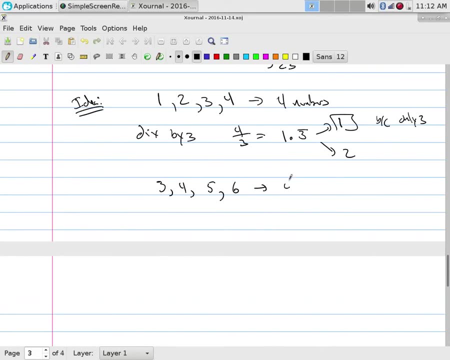 what would have happened if I would have had a different for group of four numbers? what if I would have had three, four, five and six? how many numbers do you see? that's four numbers in your div by three is four thirds, which is equal to 1.3. repeating, which is either going to be one or two. it's two because it's. 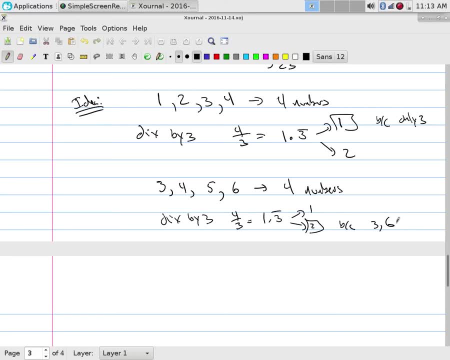 three and six. so what happens? you have this window. if the window does not perfectly match your div, what happens is if the window always has the possibility of getting both of the ends hitting, and then you get the higher number, or if both of the ends are essentially empty, you get the lower number. so as the window moves, it's like 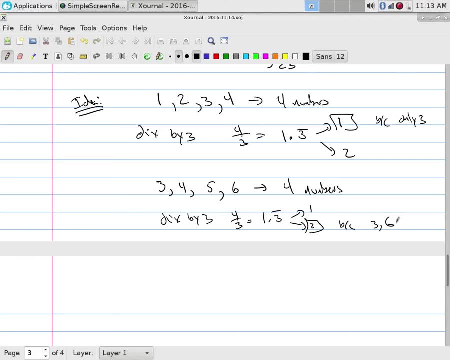 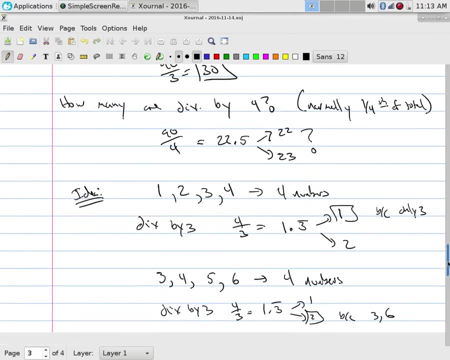 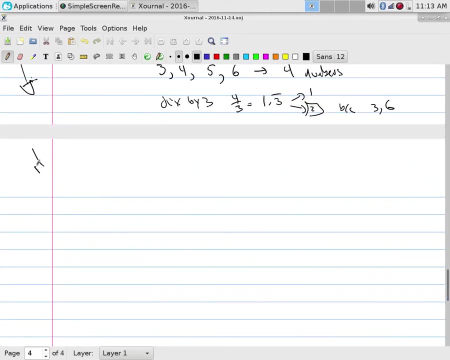 up one up now to back to one. now to back to one. so see how that idea works. think about the harder problem all the way up here. now we are doing 10, 11, 12, 13, 14, 15, all the way up to 96, 97, 98 and 99, and I say div by 4. and I found out that I was. 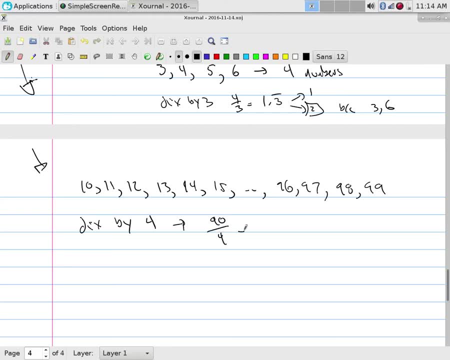 taking 90 divided by 4, and I got my 22.5. so it's either going to be 22 or it's going to be 23. the question is: which is it? where's my first div by 4, 12? that's my first div by 4. 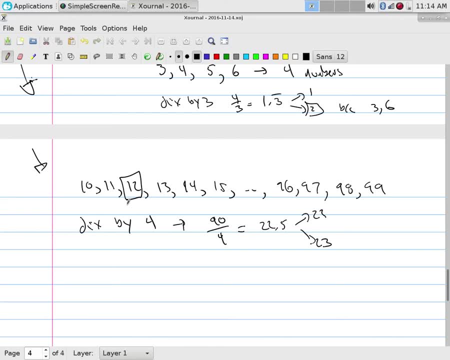 where's my last div by 4? how do you know? how did you know? because 100 is, like that's, very easy one. so 100, we knew, was divisible by four. so four in front of it, one, two, that would be a remainder. three minor two, remainder one, so it's 96. so from 12 to 96, how? 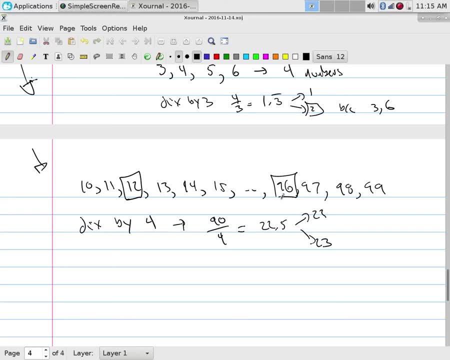 many are there. how many multiples of four are from 12 to 96. could you find out a way to do this besides counting? could you think of a way of doing this so we could start off at 12 plus how many fours is equal to 96, right? how many four steps away? 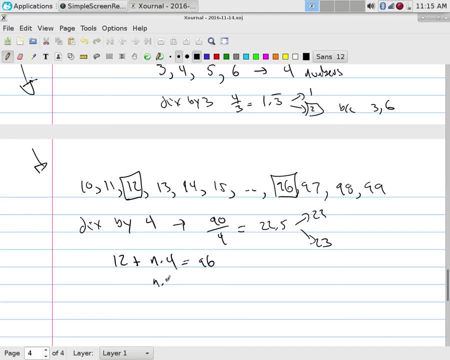 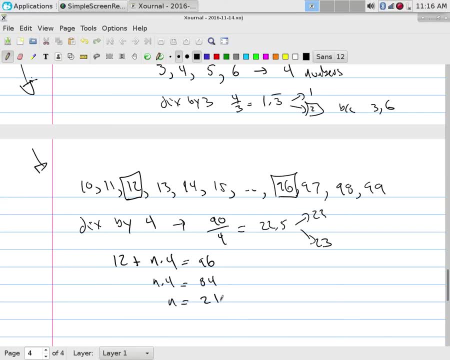 16. two steps away, is 20, 21 steps away is 97. So 96 is 21 steps away. So how many total numbers do we have 22.. So we have 21 steps away. That means that 22 is the answer. 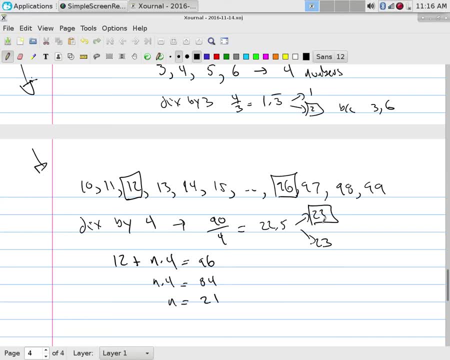 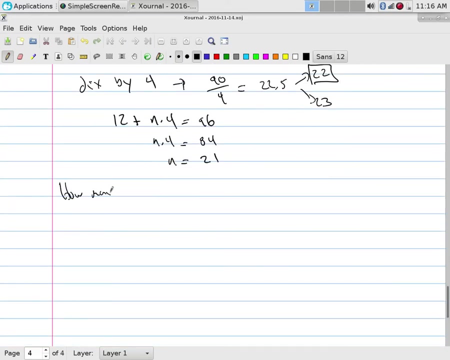 What if I found 96 would have rather been 22 steps away. What would have been your answer? It would have been 23.. Is everybody okay with that? How we got to the 22?? Here comes a fun one: How many are divisible by 2?? 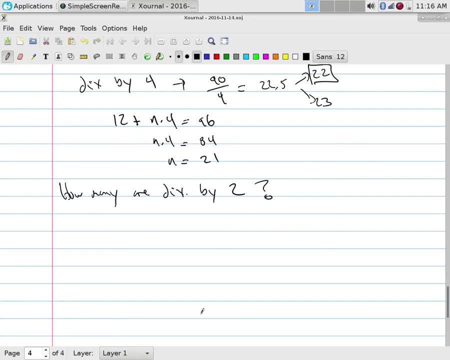 Setting up a little bit of a problem. How many total numbers were there? If it's divisible by 2, it would be about what? So it's divisible by 2.. So it's divisible by 2. It would be half. 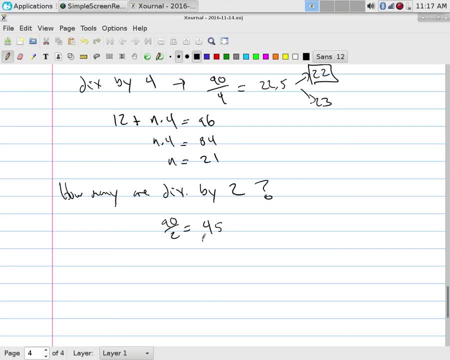 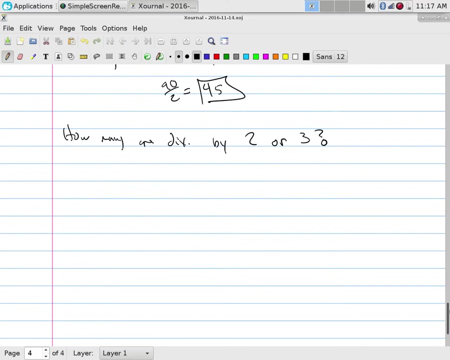 So what's 90 divided by 2?? So there's 45 that are even. There's 45 evens? How many are divisible by 2 or 3?? All of a sudden I have a word, or So it looks like we would say that the divisible by 2 or 3. 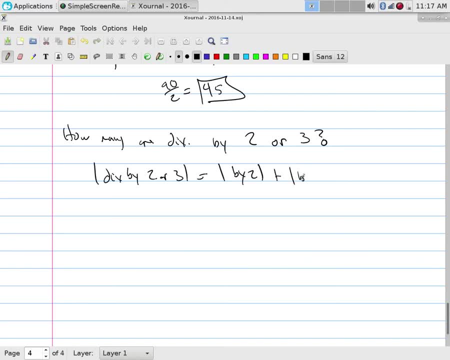 should be the cardinality of by 2 plus the cardinality by 3.. But that would only be true if they're what, If they're disjoint? But are there any numbers that when I counted divisible by 2, that I also counted when they were divisible by 3?? 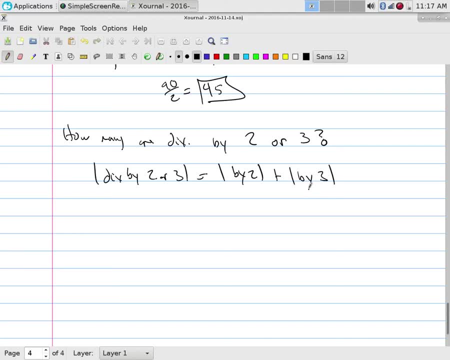 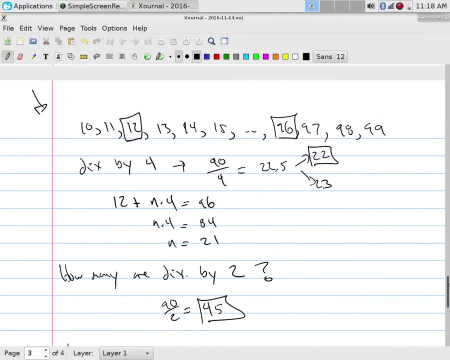 12., 12.. What else Between 10.? So we have 12.. What would be the next one? 18.. How far is 18 from 12? It's 6.. In other words, what do we have to do? 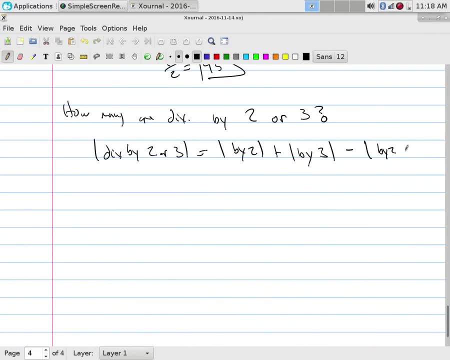 What's the intersection? And 3, which is really by what To be divisible by 2, and divisible by 3 means you have to be divisible by 6.. So the only way I can do this problem is: I need to know by 6.. 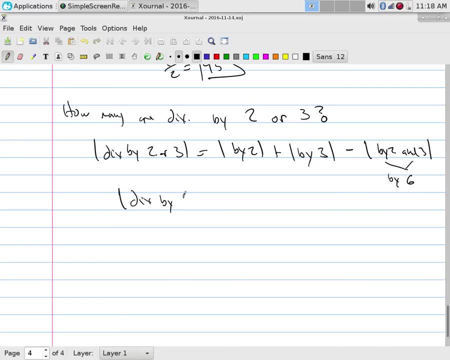 So what is the by 6?? That's equal to 90 over 6,. which is, What's 90 over 2? 45.. 45 divided by 3? Hmm, I heard, like several right now, 40 divided by 3.. 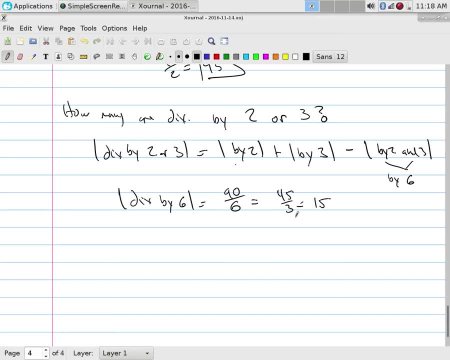 15.. My ears are not good, So what's my answer? 2 or 3 is how many were by 2?? How many by 3? 30. And then I take away 15, which is equal to 60.. 60. And then I go by 2. And it's 1 over 2, which is 4 over 3.. Right, right. So what's the answer Now? it's 1 over 2.. It's 1 over 2.. So what's the question? How many times do we have to prove what's going on? It's time to prove the answer. Tim Question time. How many times do we have to prove the answer When we get the answer to the question? Is it only 1 or 2?? Well, we'll show you in a couple of seconds. So it's a lot of numbers in terms of how many times we have to prove it. How many times. Well, it's a lot of numbers. We need to figure out the answer.